Disharge is therefore the amount of water originating as precipitation which reaches the channel by runoff, which includes overland flow, through flow and base flow. Disharge is therefore the amount of water originating as precipitation which reaches the channel by runoff, which includes overland flow, through flow and base flow. 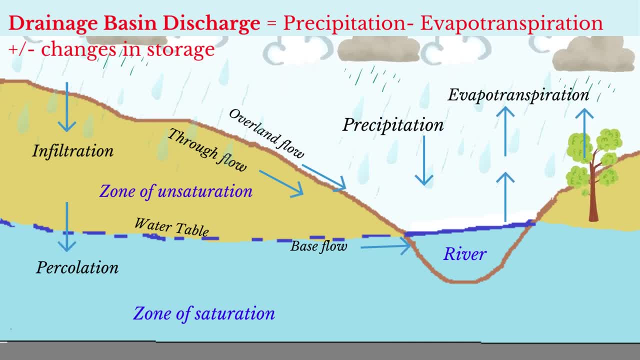 Disharge is therefore the amount of water originating as precipitation which reaches the channel by runoff, which includes overland flow, through flow and base flow. Discharge is therefore the water not stored in the drainage basin or lost through evapotranspiration. 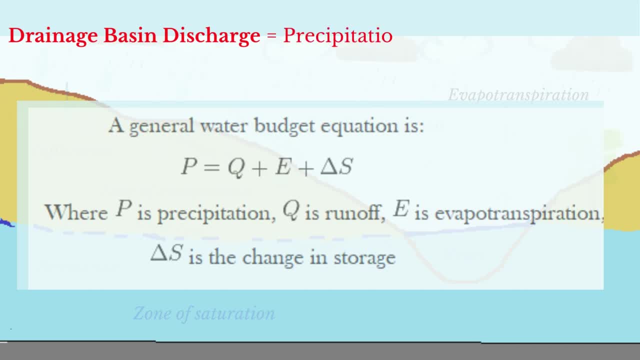 Notice how similar the discharge equation is to the water budget or water balance equation. The water balance equation is precipitation. The water balance equation is precipitation. The precipitation is equal to runoff plus evapotranspiration plus changes in storage. If you take a careful look at both equations, you will realize that discharge in the first equation is the same as runoff. 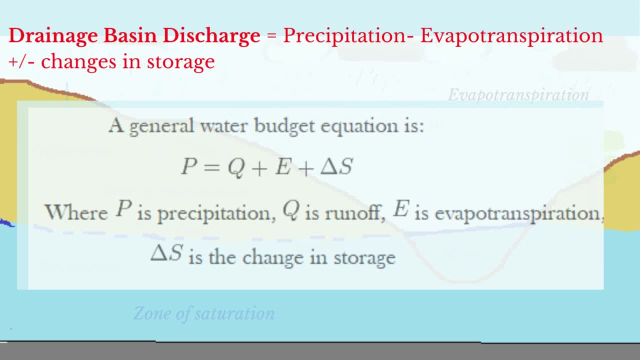 The discharge in the first equation is the same as runoff. The discharge in the second equation is the same as runoff. If you take a careful look at both equations, you will realize that discharge in the first equation is the same as runoff. If you take a careful look at both equations, you will realize that discharge in the second equation is the same as runoff. 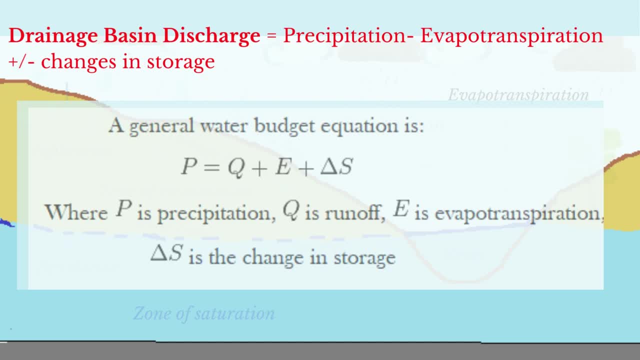 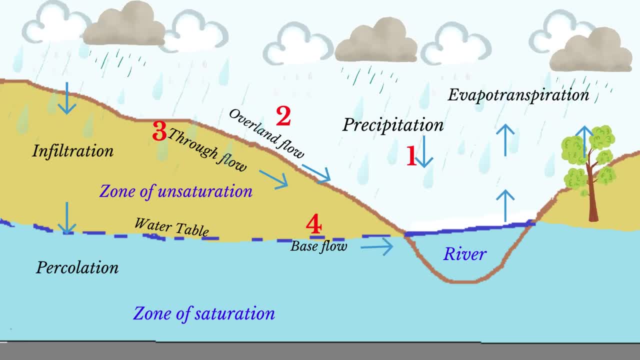 Now, the fastest way that rainfall can reach the river channel is via direct precipitation. The next fastest route is water flowing over the surface as overland flow. This is followed by the next route, where water flows over the surface as overland flow. This is followed by the next route, where water flows over the surface as overland flow. 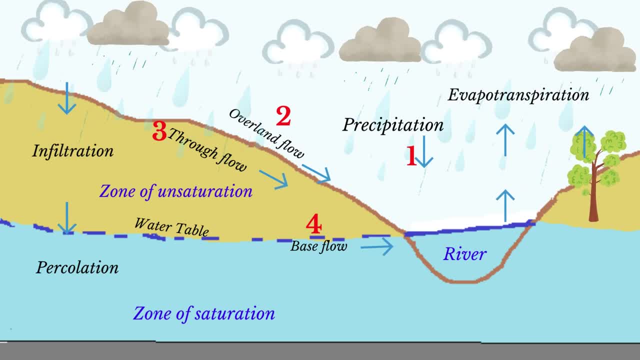 Water first infiltrates into the ground and then flow sideways as a through flow before getting to the channel. The slowest route is where the water infiltrates into the ground, then goes even further down by percolation and then flow sideways as base flow. 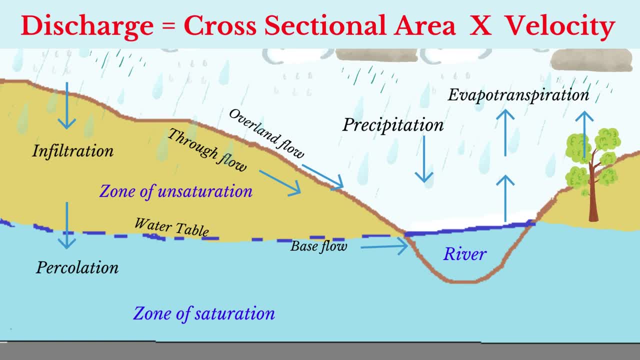 Whatever the route that is taken by the water, eventually it gets to the river and begin to flow through the channel at a certain velocity, which is controlled by the channel shape and roughness Within a river channel. discharge can be expressed as the equation: 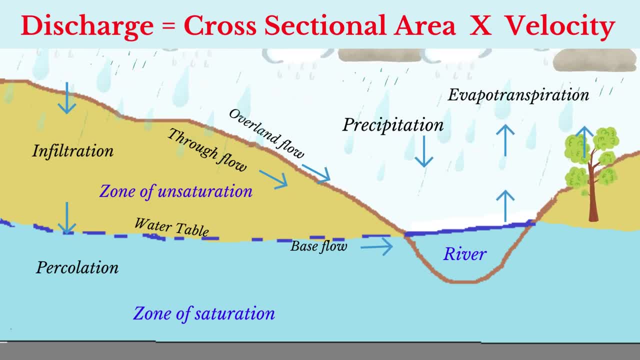 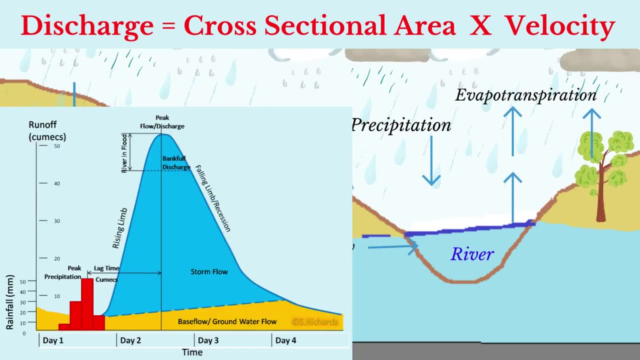 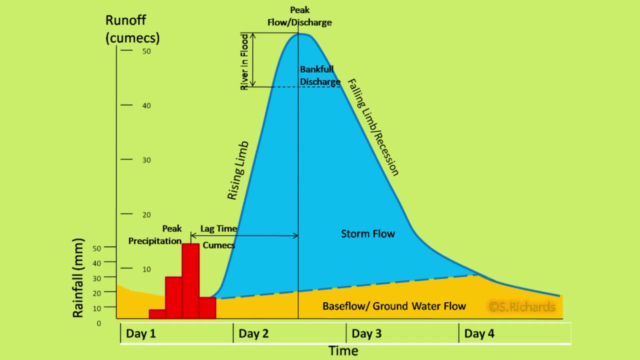 Discharge is equal to cross-sectional area multiplied by velocity. To show the variation of river discharge with time at a particular point within the channel, a storm hydrograph can be drawn. A storm hydrograph is a graph. A storm hydrograph is a graphical representation of water output from a watershed, typically presented as a stream flow time series. 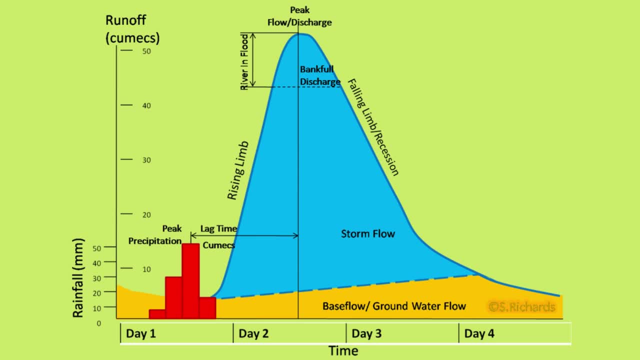 The graph shows the effect that a rainfall event has on the discharge of a river. It also shows how the drainage basin responds to a period of rain. The main elements of the graph are the rising limb, the falling or recession limb, The lag time, the base flow, the storm flow, the bankfull discharge, as well as the peak discharge. 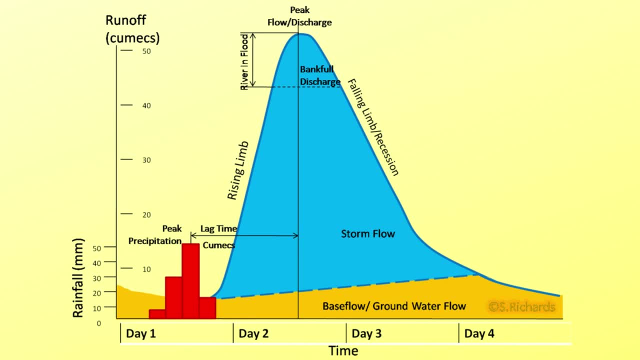 The base flow is the contribution made to the river by groundwater. The storm flow is water that arrives in the river channel. The bajer, the start of the stream flow, carries water in a river, the fool, The rising limb skipped as above, plus the peak discharge increases from a water-flowing river to a vertical flow of water. 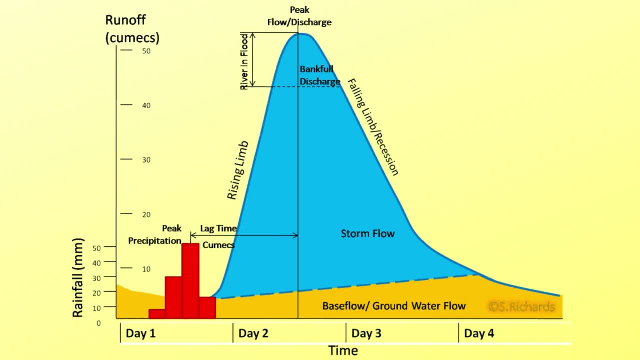 which is the wind track, the more likely it is for a flood to occur. The falling limb, or recession limb, shows the river as the level begins to fall. If a secondary rainfall event occurs, the falling limb could be interrupted. The bankfull discharge, as the name suggests. 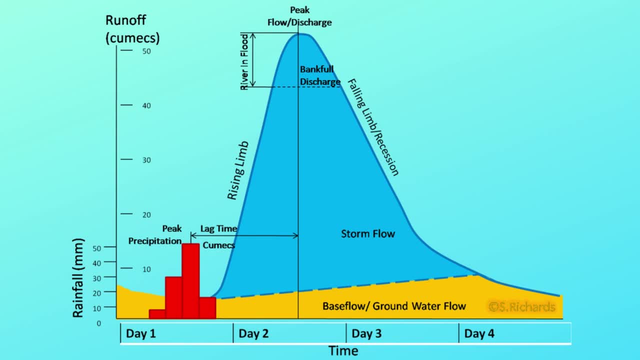 is where the water reaches the top of the channel. Peak discharge is the maximum amount of water in the river channel, So the peak discharge could be lower than the bankfull discharge, it could be at the level of the bankfull discharge or it could be greater than the bankfull discharge. 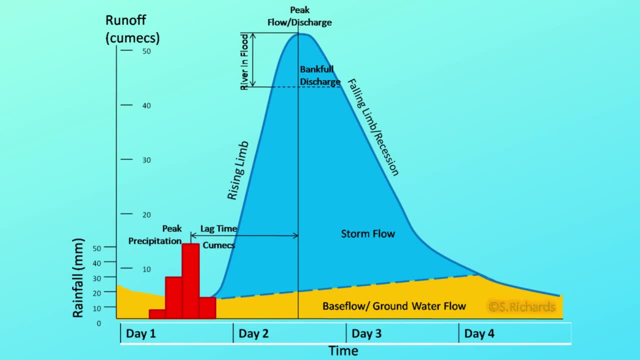 If it is greater than the bankfull discharge, a flood will occur. This is because the water has overtaken the river banks. The term lag time refers to the amount of time between the peak rainfall and the peak discharge in the river. The shorter is the lag time, the faster the water reaches the channel. 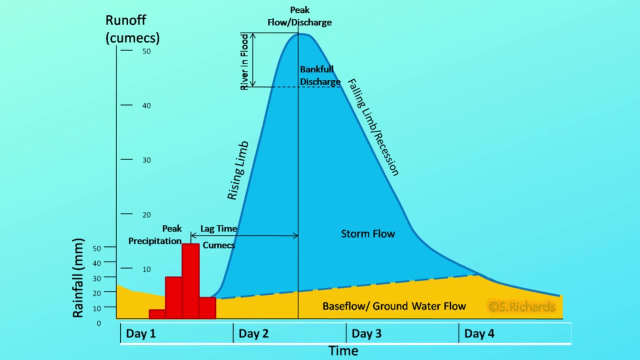 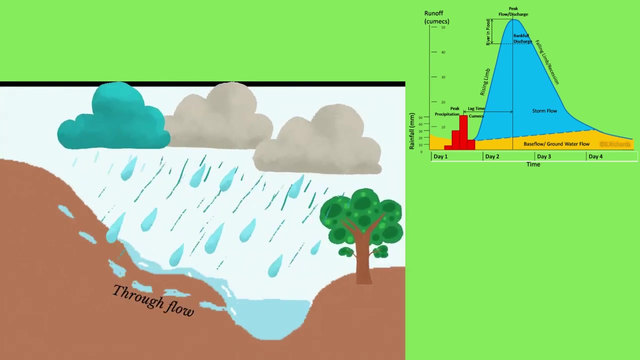 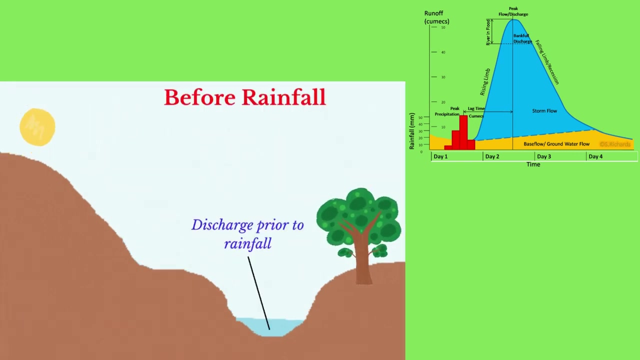 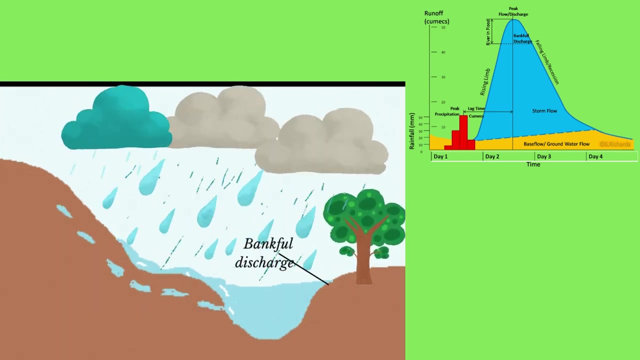 and therefore the faster the level of the river, Thus the more likely it is for a flood to occur. The animation shows that prior to the rainfall event, the discharge is low. When the rainfall begins, the water level starts to rise slowly. 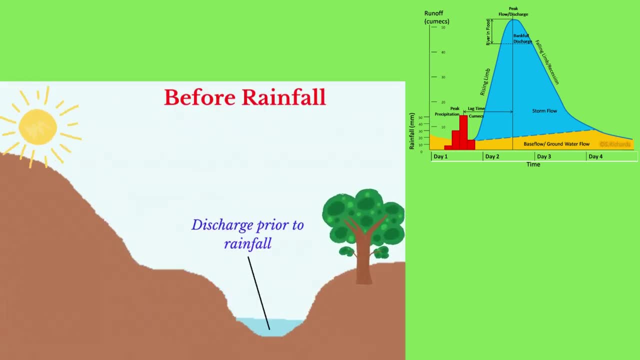 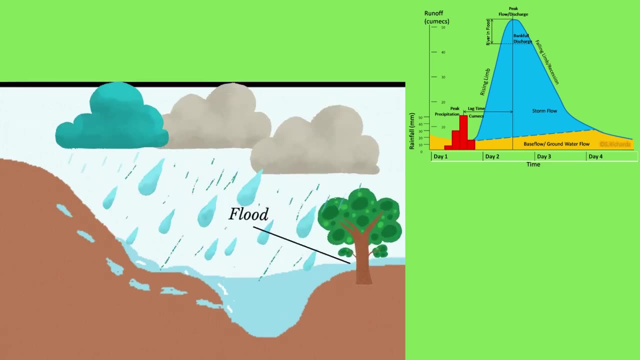 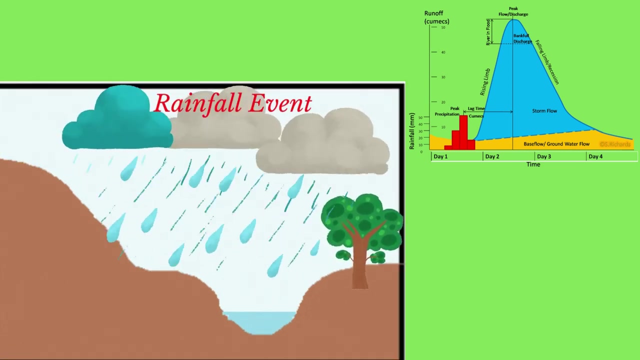 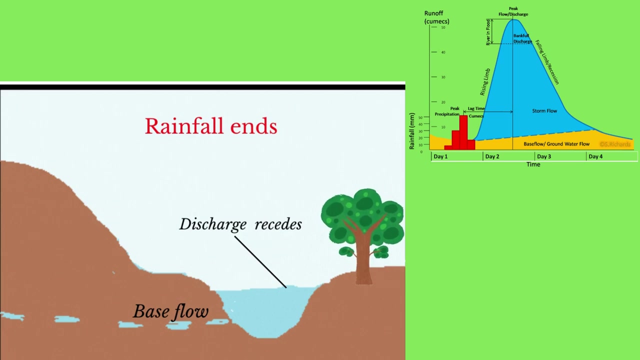 because of the direct feed of the rainfall, Soon water begins to rise even more as water is added to the channel by overland flow. As time passes, more water will be added to the channel via through flow At a certain point in time. 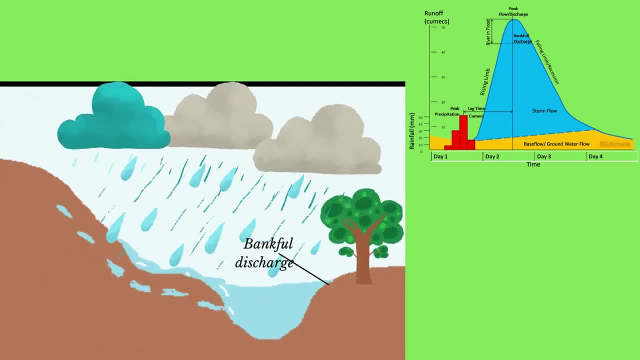 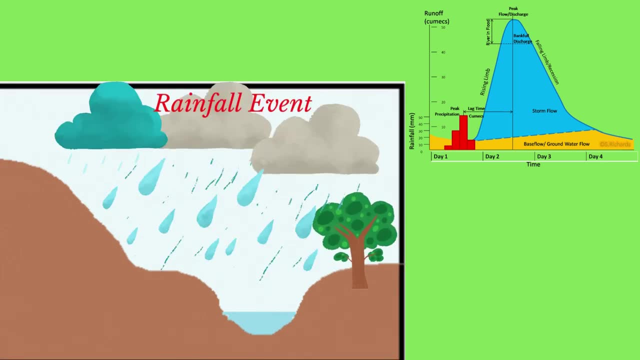 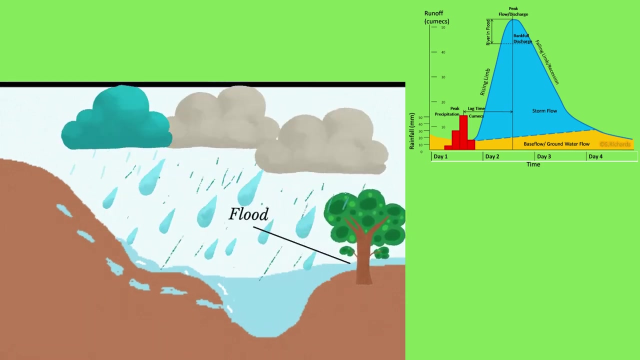 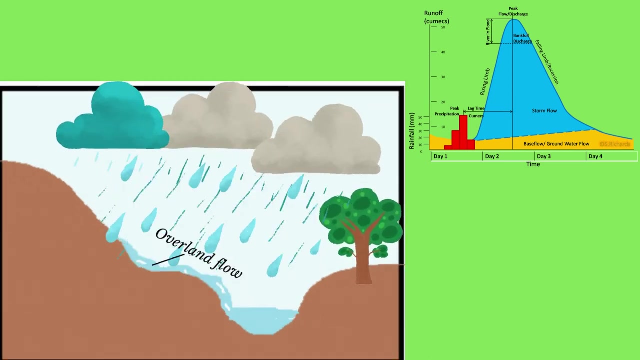 the discharge may rise to the point where it reaches the top of the channel and is therefore at bankfull discharge. When the discharge surpasses this level, flooding begins. After the rainfall ends, the water starts to recede. However, after the rainfall ends, the water starts to recede. 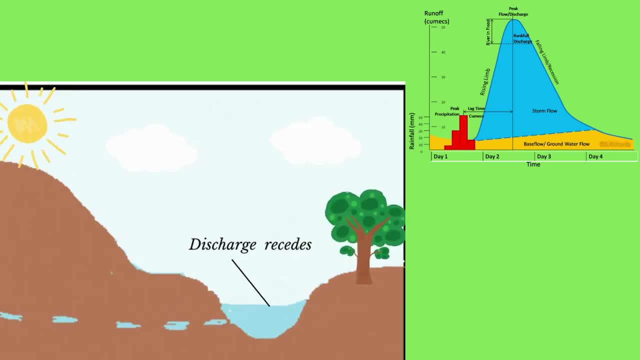 However, after the rainfall ends, the water starts to recede. However, after the rainfall ends, the water starts to recede. This is a slow process, as the water continues to be added to the channel. as the water continues to be added to the channel. 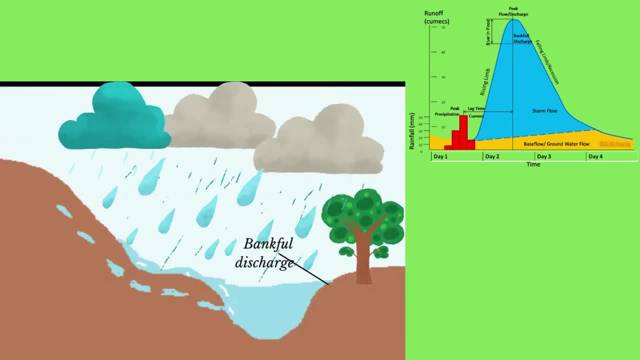 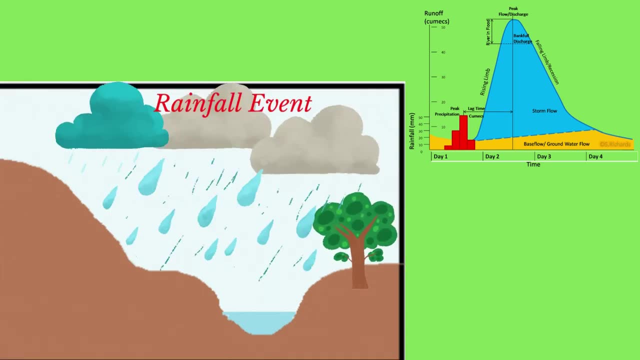 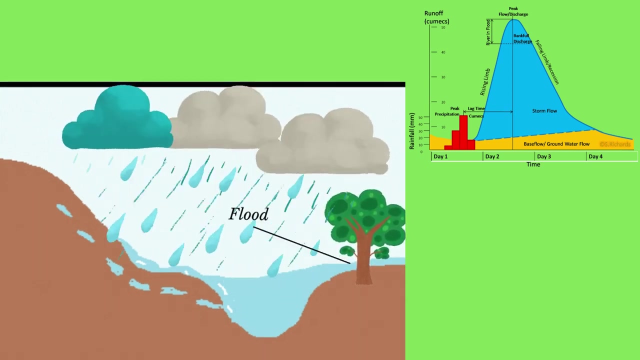 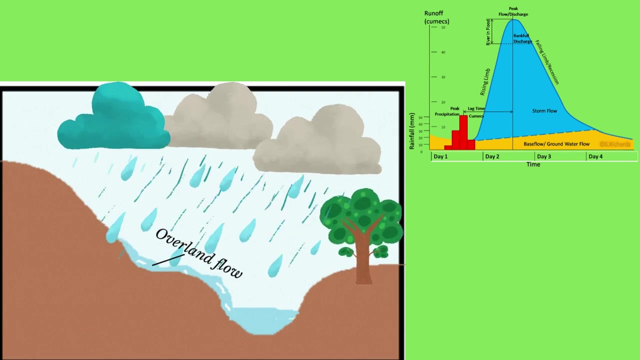 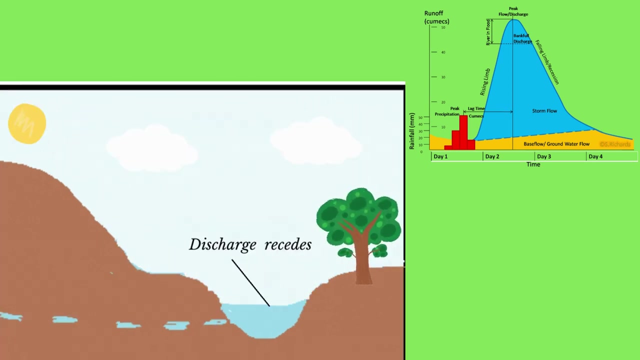 by the slower process of the base flow. All of this is what is represented by the hydrograph. The histogram is this histogram Some of the media have paraphrased. it represents the rainfall event and the highest column of the histogram shows the peak rainfall. 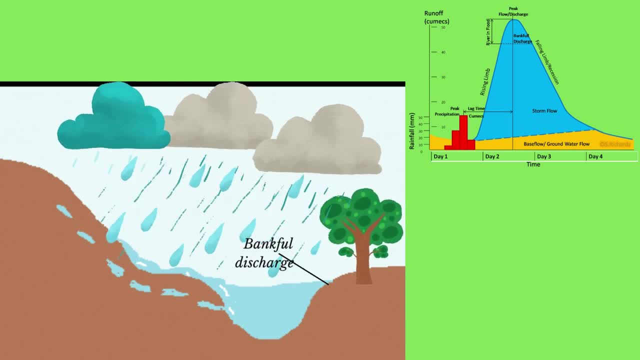 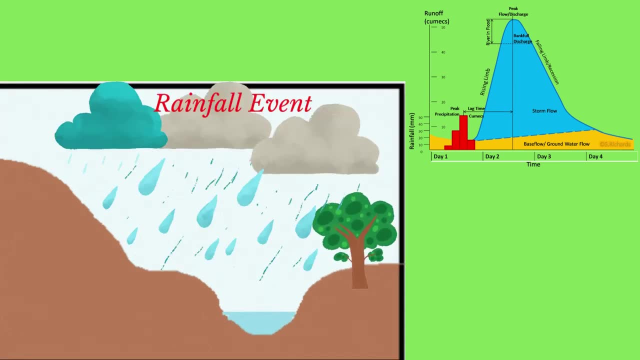 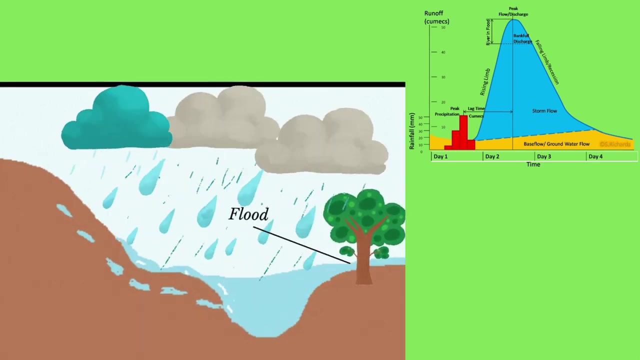 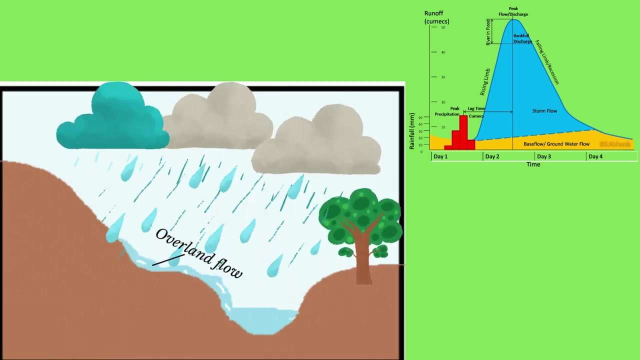 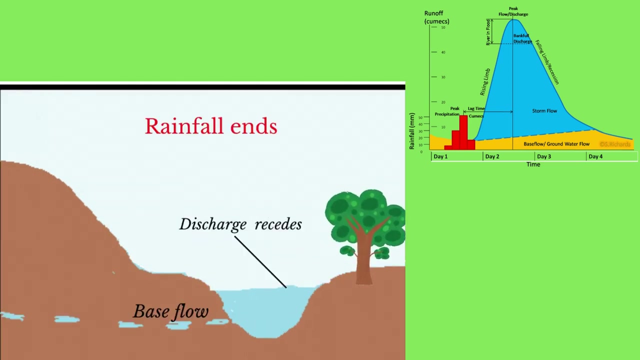 The discharge is being shown by the line graph and the highest point of the line graph is showing the peak discharge. The part of the line graph that ascends towards the peak discharge is our rising limb, and where the line descends from the peak discharge is our falling limb. 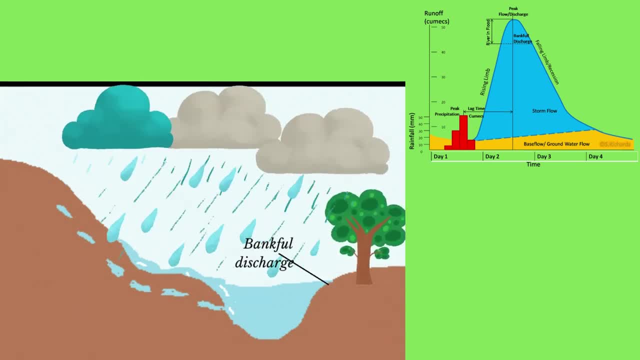 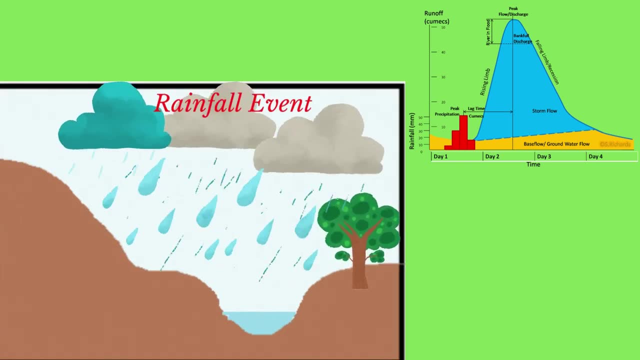 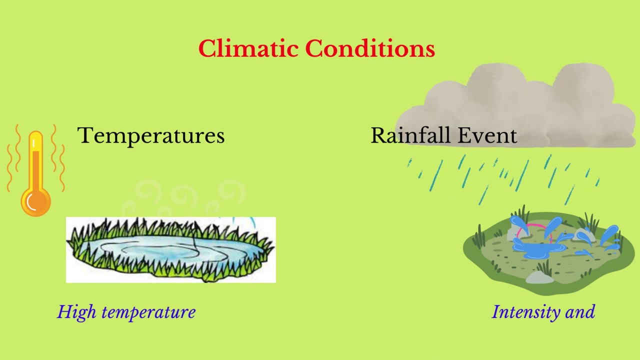 Notice that the distance from the peak discharge is being shown by the line graph. Notice that the distance from the peak discharge is being shown by the line graph. To the peak rainfall is the lag time Now. the shape of the storm hydrograph varies based on a number of factors. 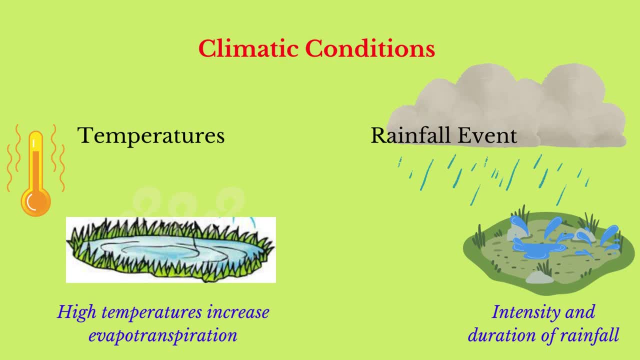 These factors may be climatic factors, It may be drainage basin characteristics, Or it could also be human activities and human structures. Let's first look at climatic conditions. Low temperatures can cause a soil to freeze, causing it to act as an impermeable layer. 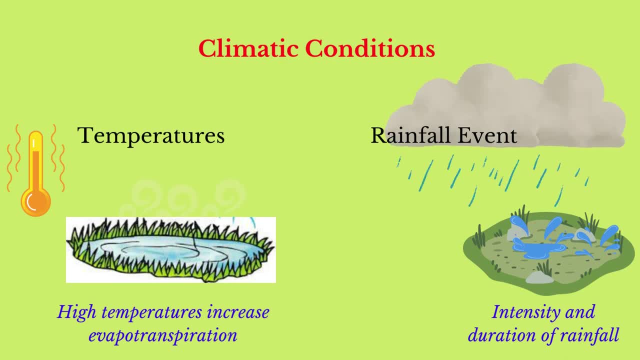 This restricts infiltration and increase overland flow. As such, there's There will be a shorter lag time. Where temperatures are high, the rate of evapotranspiration will increase, reducing the amount of water that flows into the river as overland flow. 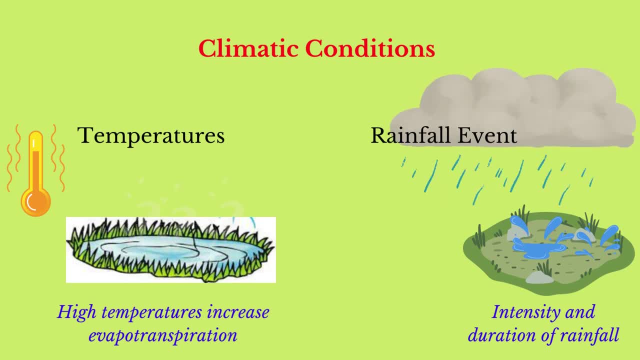 In terms of precipitation, high-intensity rainfall reduces infiltration and increases overland flow. The rainfall of long duration will eventually cause the soil to be saturated, And when the soil becomes saturated, infiltration will be restricted. When infiltration is restricted, more water will flow as overland flow. 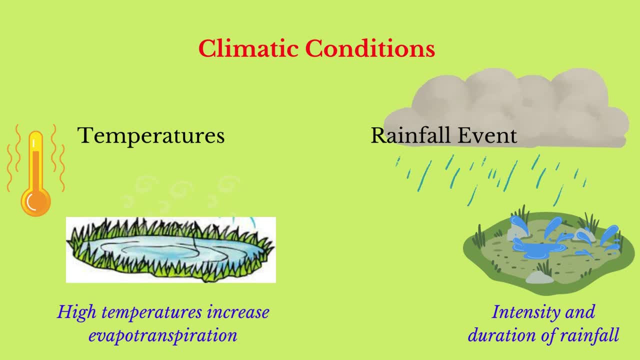 Snow is another type of precipitation. When the snow event has just occurred, most of the water will be held in storage, But when there is a snow melt, The water will generally flow quickly over the frozen ground that now behaves impermeable towards the river channel. 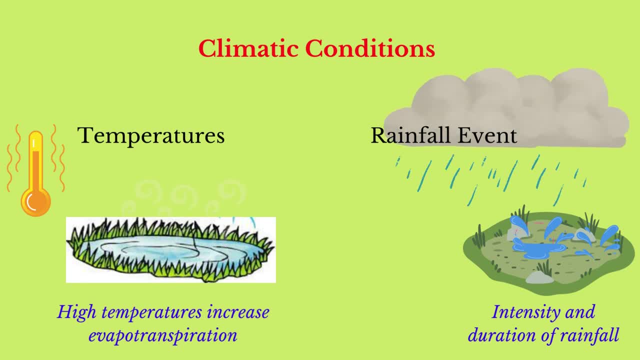 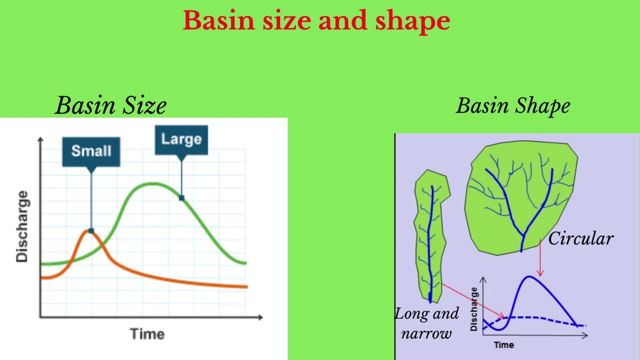 Remember, the faster the water gets to the river channel, the shorter is the lag time, and the shorter is the lag time the steeper will be the rising limb. Redalah is less likely toosa into the ground than 안녕하세요 is. 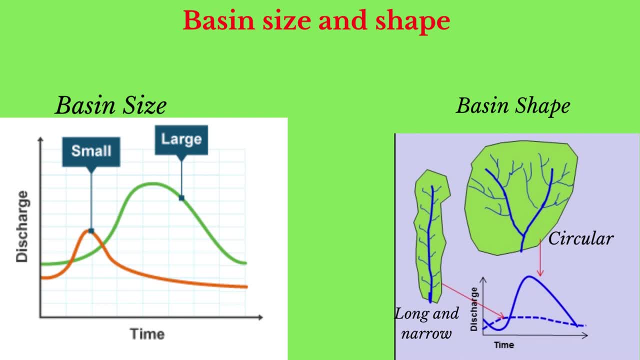 Now onto drainage basin characteristics: The size and the shape of the drainage basin. The size and the shape of the drainage basin will also affect the shape of the storm hydrograph. The smaller the basin, the less time it takes for the water to命pun yin. 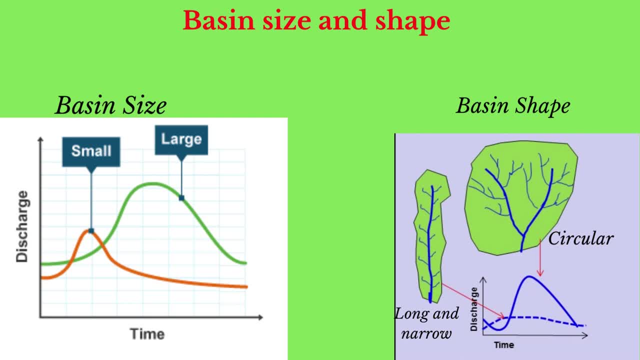 estadio, which is cloud waters Now for layer. As shown on the slide, Thousands ofTalkers- there are thousands of people working in this garden- takes for the water to get to the river channel. therefore, the shorter will be the lag time and 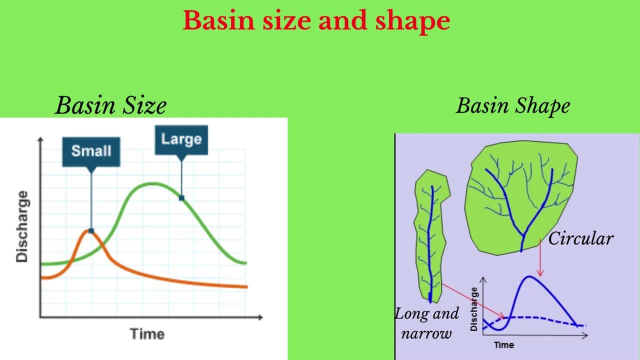 the steeper the rising limb. the larger the drainage basin, the longer the distance the water will have to travel. therefore, the longer will be the lag time and this will result in a gentle rising limb in terms of shape. when there is a circular drainage basin, the water tends to 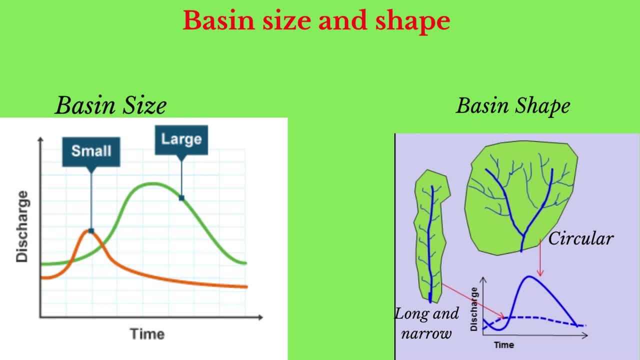 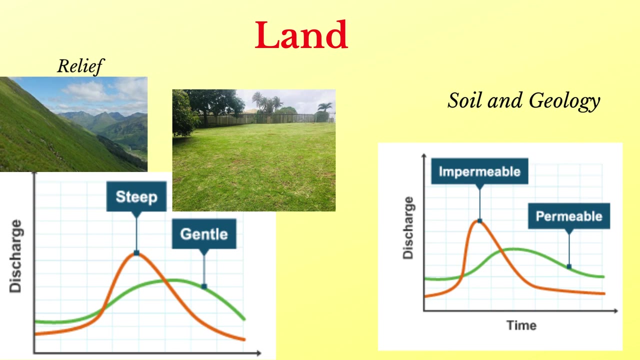 get to the channel faster. in a long and narrow basin, water tends to take a longer, longer time to reach the channel. the relief of the land is another factor that influences the shape of the storm hydrograph. the steeper the land of the drainage basin, the faster the water will flow. 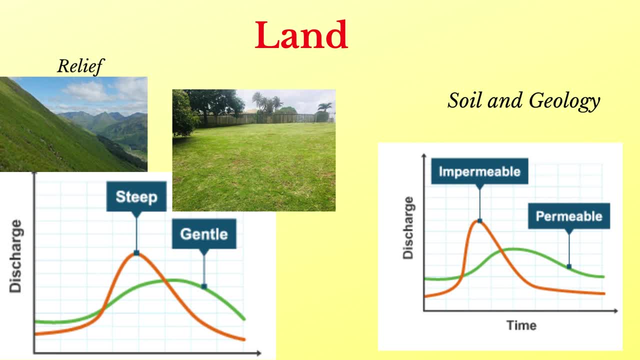 which means a shorter lag time and a steeper rising limb. if the relief of the land is either gentle or flat, there will be more infiltration and therefore a longer lag time. in terms of geology, permeable rocks will encourage infiltration and therefore will cause a longer lag time and a gentle rising limb. 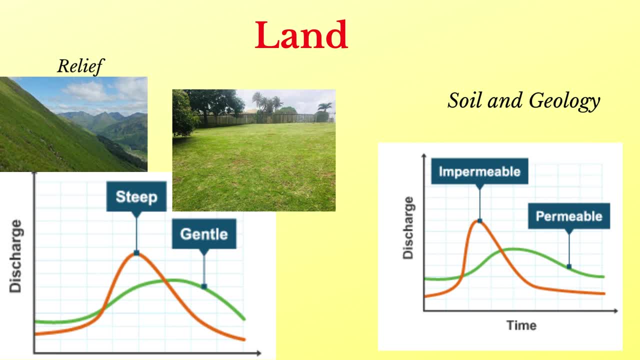 if the rocks are impermeable, on the other hand, overland flow will increase, lag time will be shorter and there will be a steeper rising limb. this is also true of the soils. so soils like sand with larger pore spaces will encourage infiltration, and this will this will cause a longer lag time. soil such as clay soil. 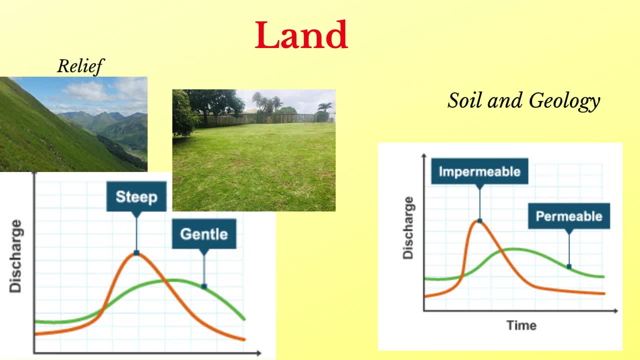 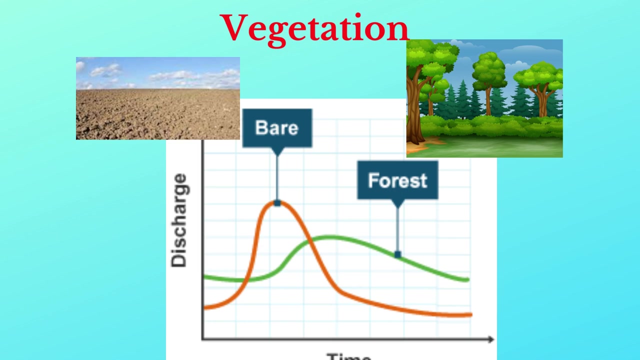 with smaller pore spaces will result in greater rates of overland flow, shorter lag time and a steeper rising length. vegetation is important as it reduces. vegetation is important as it reduces discharge. this is because the vegetation often intercepts precipitation and adds to the rate of evapotranspiration. 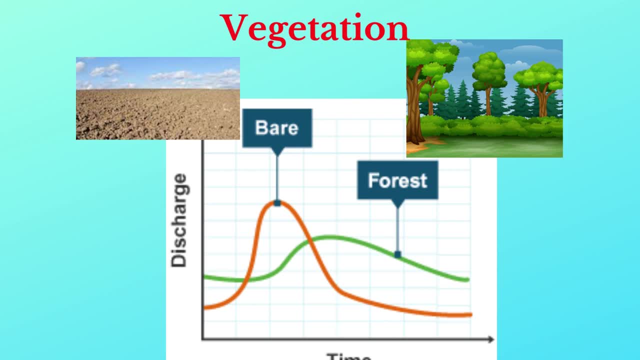 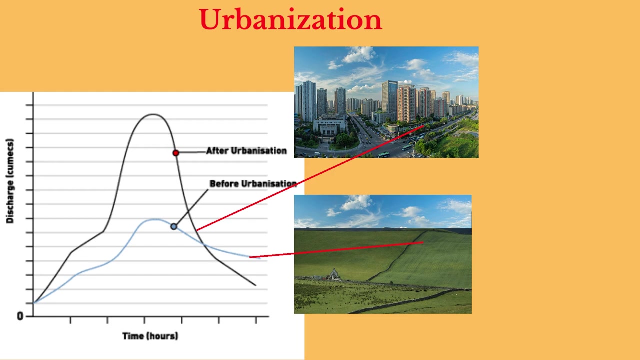 the roots of plants also take up water, reducing through flow. thus the greater the vegetation, especially trees, the greater the lag time and the gentler the rising limb. Urbanization helps to alter the hydrological cycle, For example concrete and tarmac form. 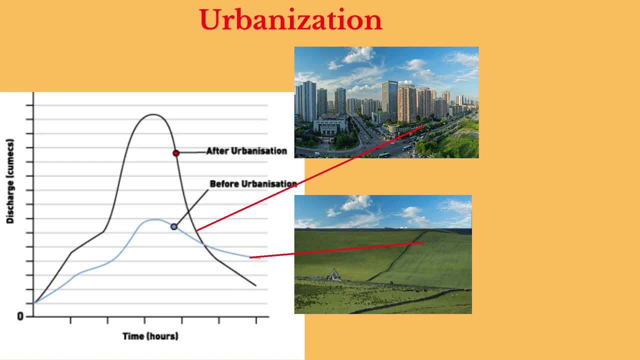 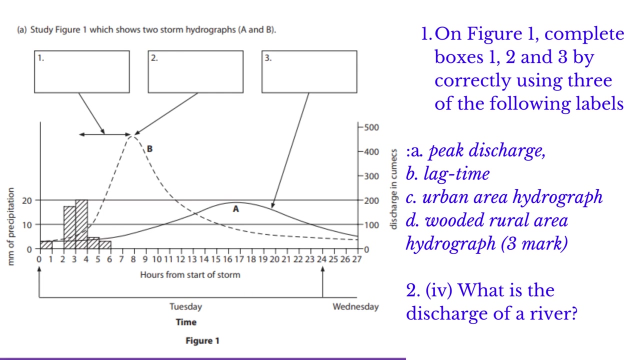 impermeable surfaces, creating steep rising limb because of the shorter lag time. Buildings also contribute to interception. Okay, so, as I come to the end of this video, I am going to leave you with a past paper question. This time, this past paper question is not from the CAPE examination, It is actually a GCSE past paper. 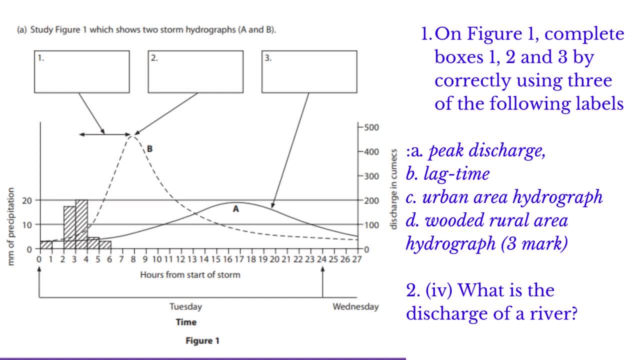 question. It requires you to label a diagram showing two storm hydrographs. All right, so let us examine the diagram. Notice that number one would be the lag time. As you notice, the arrow is drawn from the peak rainfall to the peak discharge. 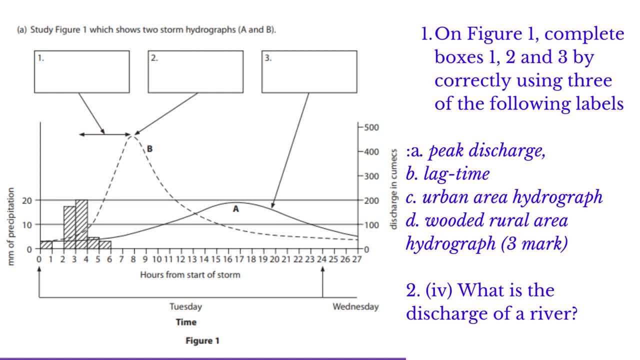 Number two would be the peak discharge, And then that leaves two more options for number three. First option is urban area hydrograph, And the second option is wooded rural area hydrograph. Now we know that if it is an urban area, lag time is going to be short. 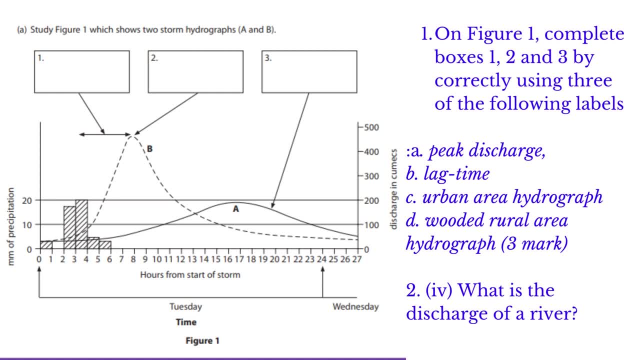 And if the lag time is short, we are expecting the rising limb to be steep and the peak discharge to be high. So since number three is pointing to the lower and gentler hydrograph, The best or the better option would be the wooded rural area. Since the presence of the country And the best and more abundant Middlale and the rural area would be. the one said, in the current scenario which is running in the area high strateklich och idag danke und wichtig pathway- I liegt unter La Hане- Particularly fluffy HC dumerik, Norden fl. precio zeigt, der wieder sicher bei schwes haben Sie entsprechend dann der слulty Ausstראלte Yahige Höhe von Back ideia er. 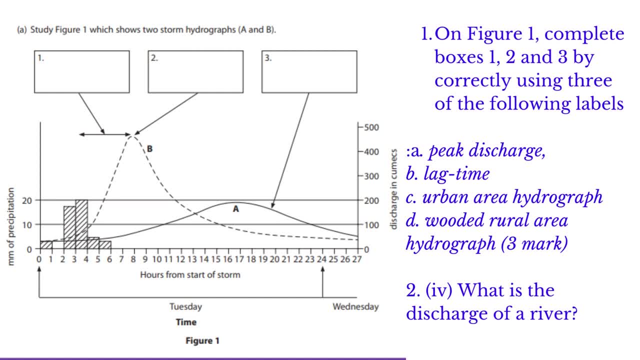 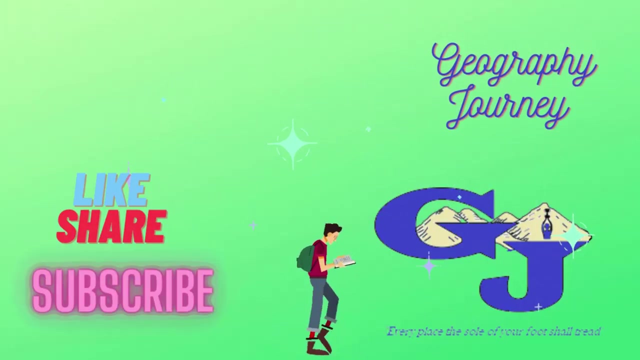 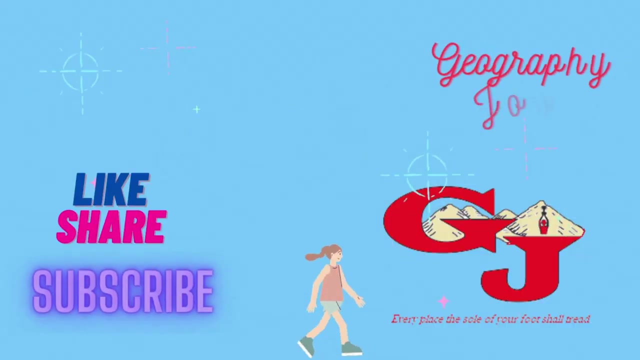 the vegetation would mean that there would be less water going into the river channel. All right, The second question is simply asking you to define the discharge of a river. OK, so I hope that this was beneficial to you. I encourage you to share this video with someone who would also appreciate the content. 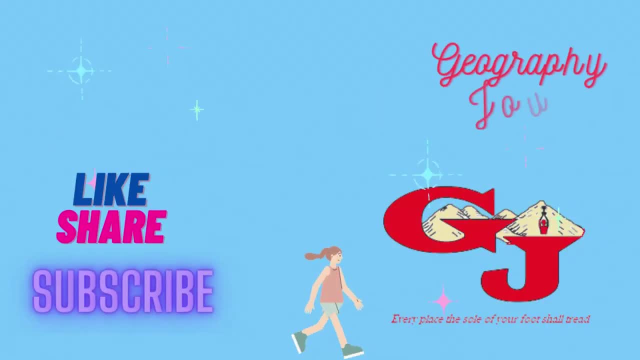 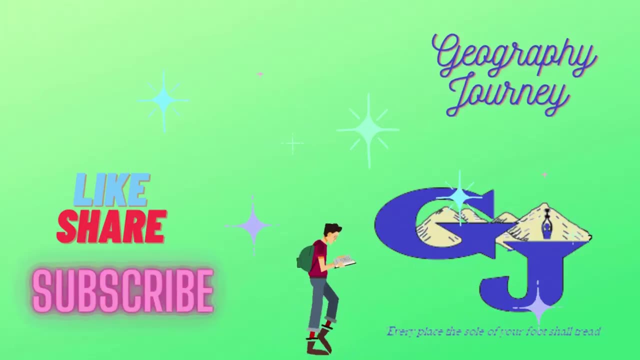 Go ahead and give me a like if you benefited from it, and definitely subscribe. Thank you.